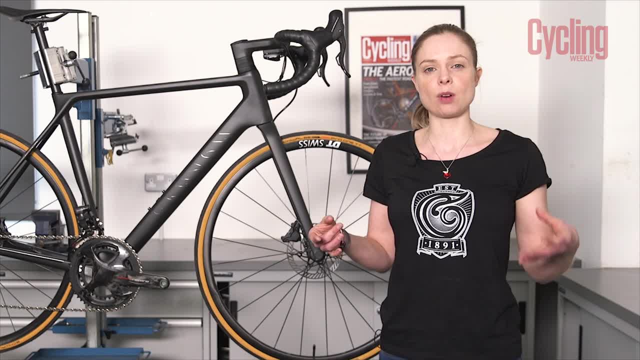 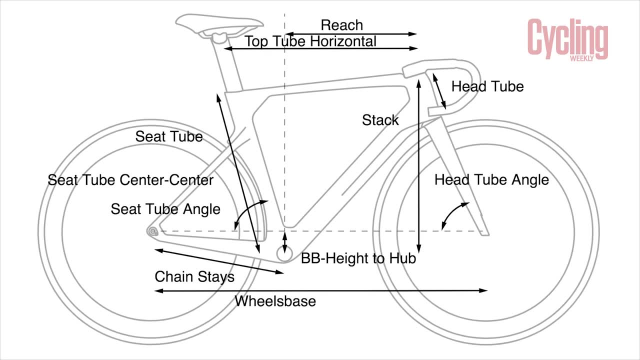 handling, because you want to determine if this is the right bike for you. The numbers you're going to look at are stack and reach, wheelbase relationship between the front centre and the rear centre, particularly the chainstays. also the head angle and trail. We're going to look at all. 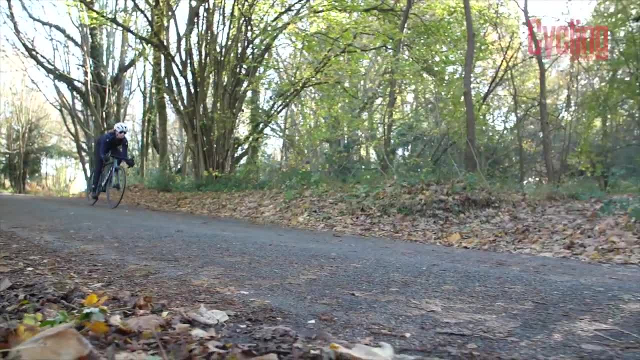 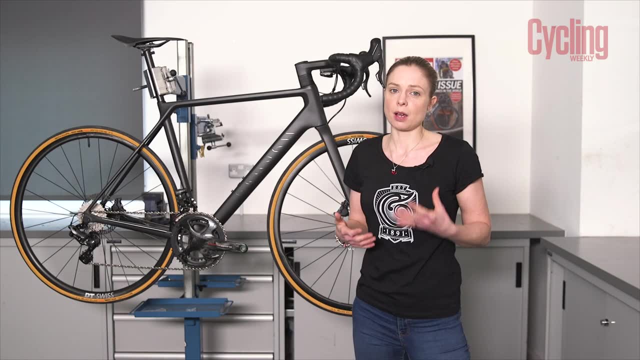 of those in this video. So once you've chosen a bike based on handling, then you're going to look at a bike based on fit, but the two really do need to interact. Be honest with yourself about the kind of rider you really are, about your strength, about your performance, about your 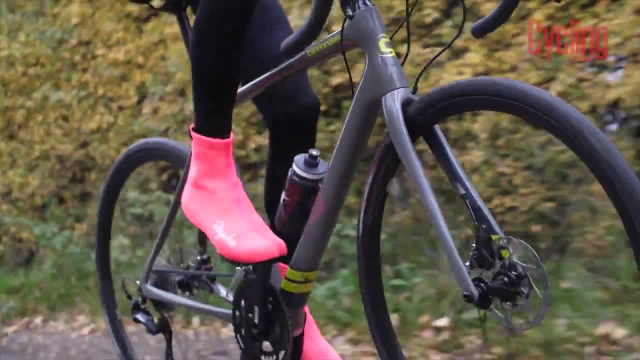 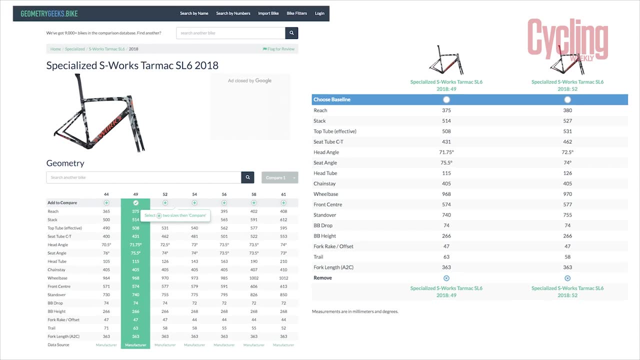 flexibility and the sort of speed you're going to be riding on, as well as the kind of roads you're going to be riding on. Now, if you are comparing a bike that you currently have with a bike you are considering buying, there are some really really useful websites out there, So it's 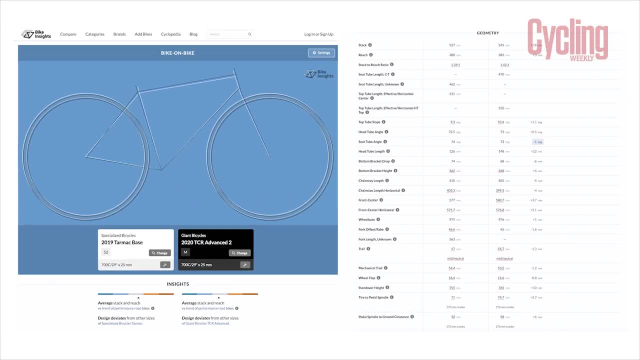 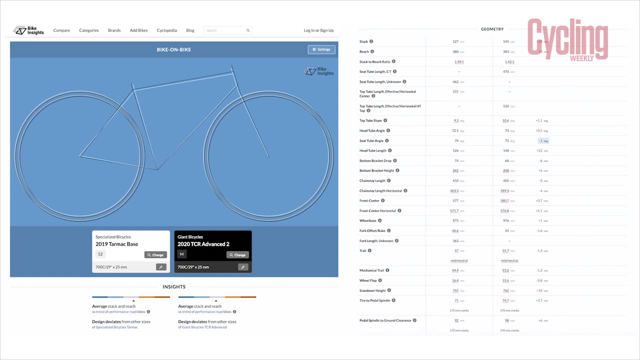 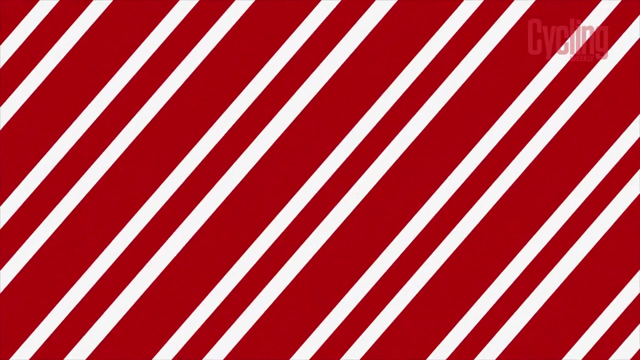 geometrygeeks and bikeinsightscom. Both of those include huge databases of various different bicycles and have all the geometry details so you can compare different bikes. So stack and reach is relatively new in terms of bike geometry charts. However, there's a very, very 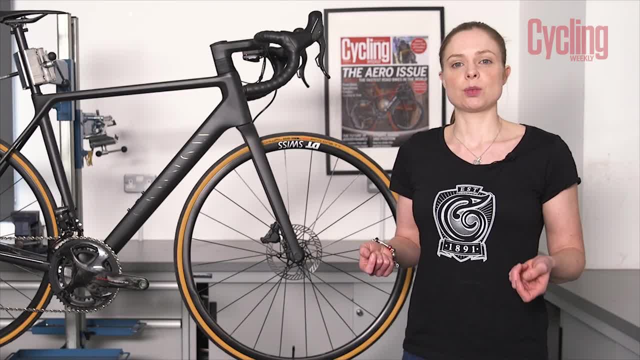 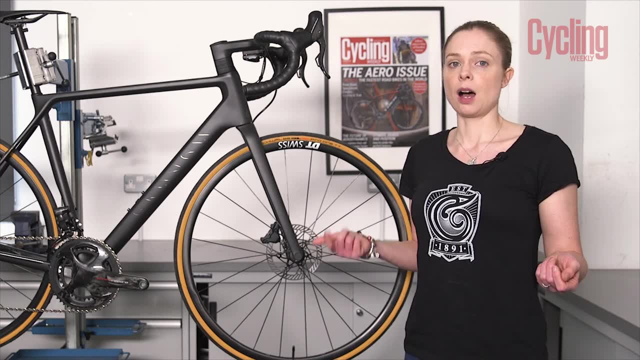 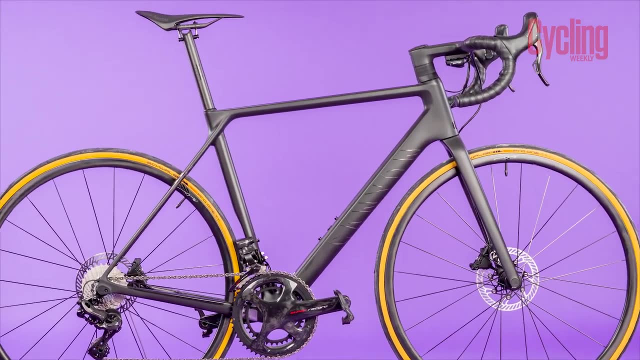 good reason for its emergence. In the past, brands would use top tube and head tube as a marker of how aggressive so long and low, or relaxed, high and short- a bicycle was. The problem with these metrics is that top tube could be measured from various different points. You could 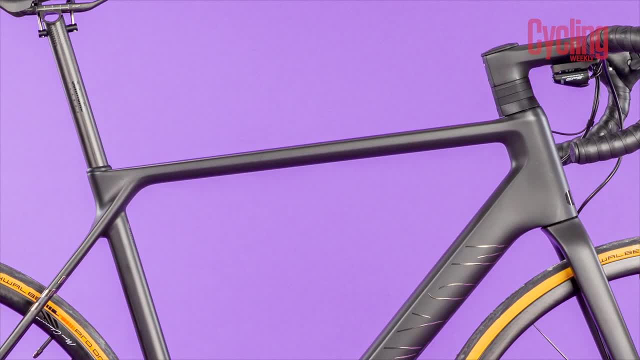 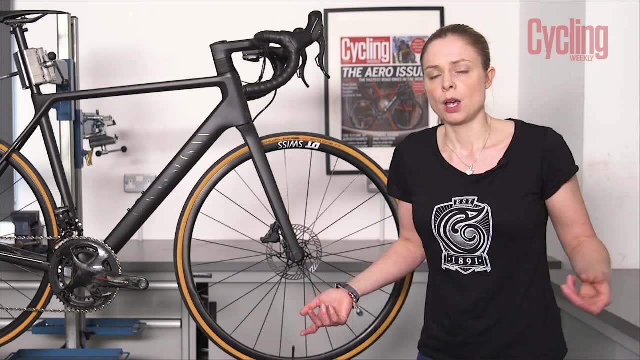 have effective top tube or centered center top tube or center center top tube or center center top tube or actual top tube, and it was never entirely clear which brand was using which metric, which made them not very comparable. The problem with head tube is that fork lengths. 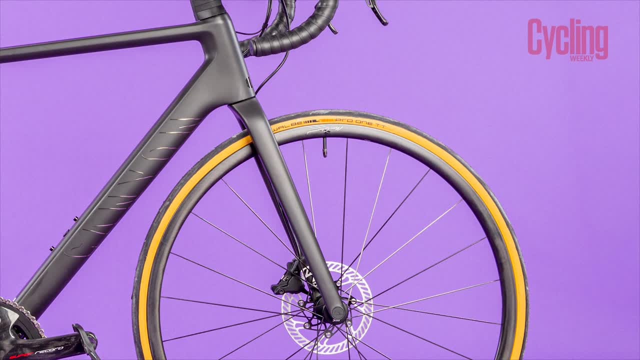 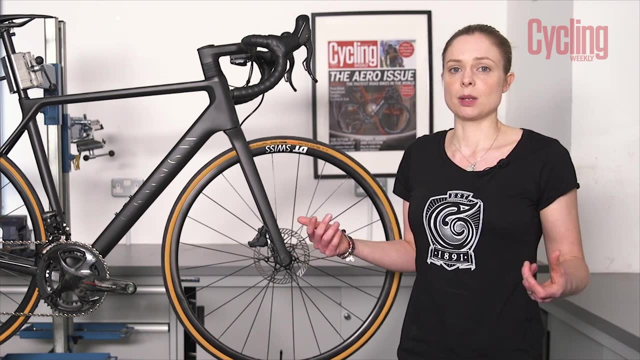 now vary quite a lot, in part because of the emergence of disc brakes and also tire clearance as well. So neither of those metrics were actually particularly useful for customers. So now we use stack and reach. So in order to explain this, I'm gonna need the post-production guys. 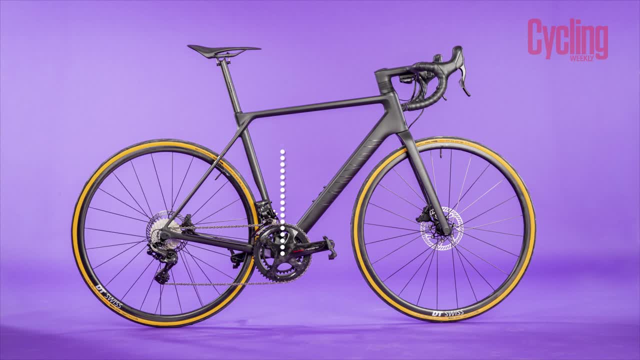 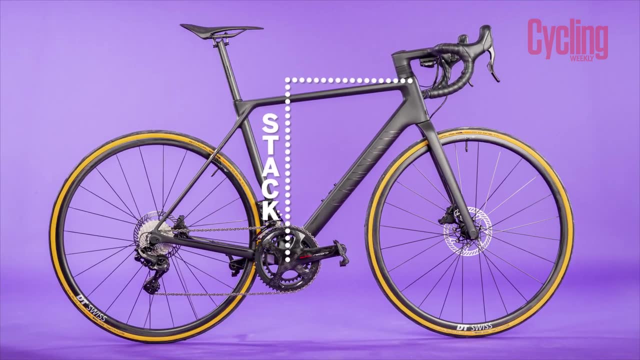 to draw some fancy lines on a bicycle Stack is the vertical distance from the center of the bottom bracket to the central point at the top of the head tube. Reach is the horizontal distance from the center of the bottom bracket to the middle of the head tube. 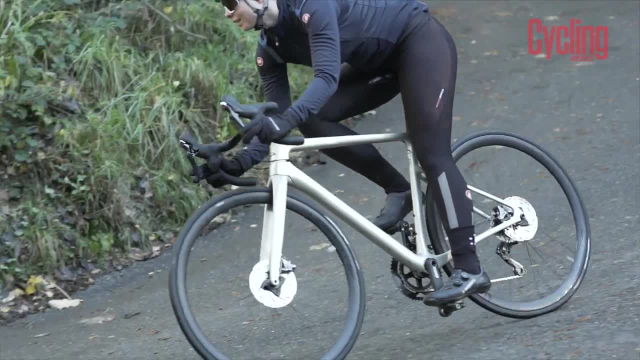 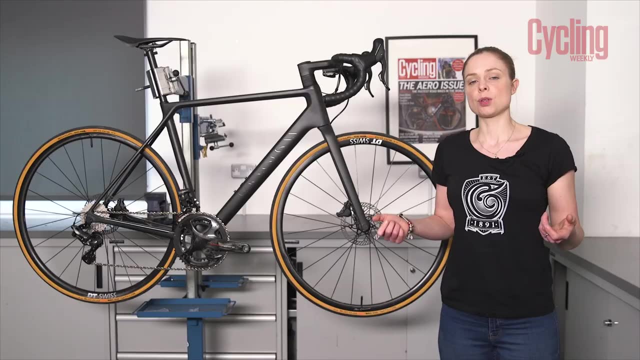 So a long reach and a short stack will put a rider in a position that feels aggressive and fast. They'll also be more aerodynamic, which is why it's often favored by racers. Of course, in order to maintain that position, you need to know that you have the flexibility. 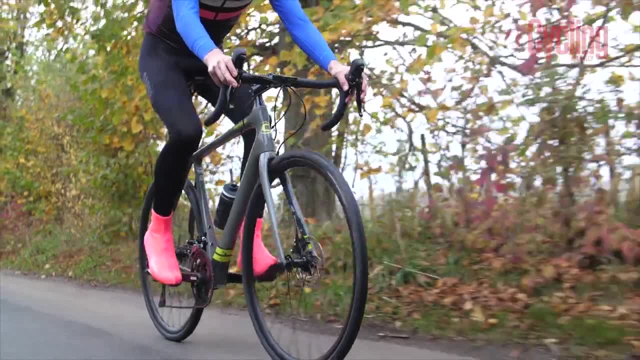 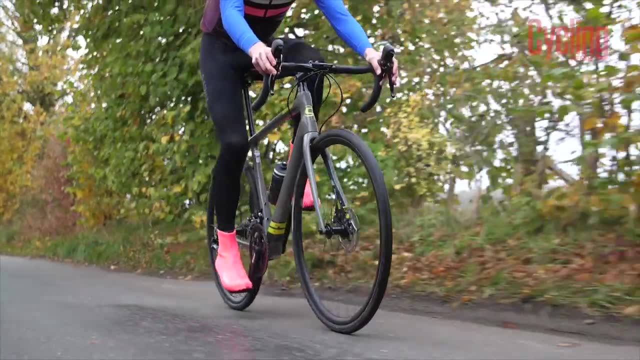 and the strength to stay there without getting injured. A shorter reach and a higher stack will feel much more comfortable and will suit riders that are gonna be out all day riding, usually at slightly slower speeds, For example, a 56 centimeter specialized tarmac. 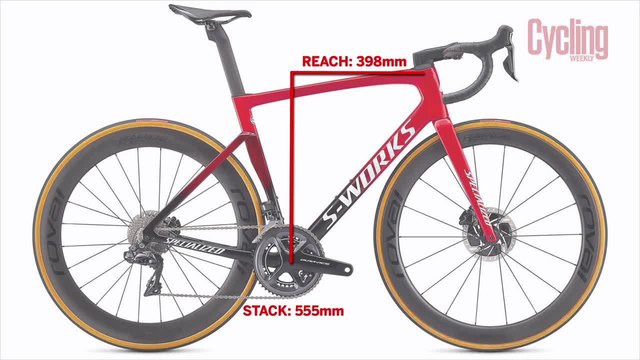 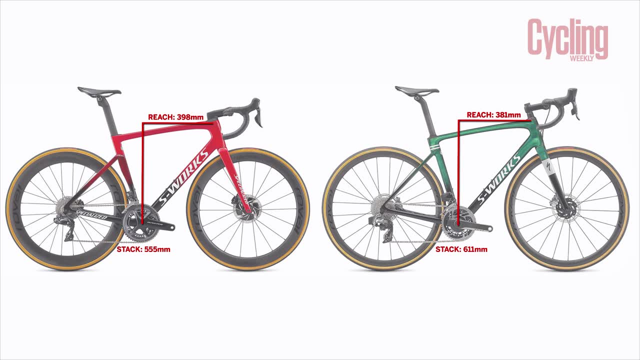 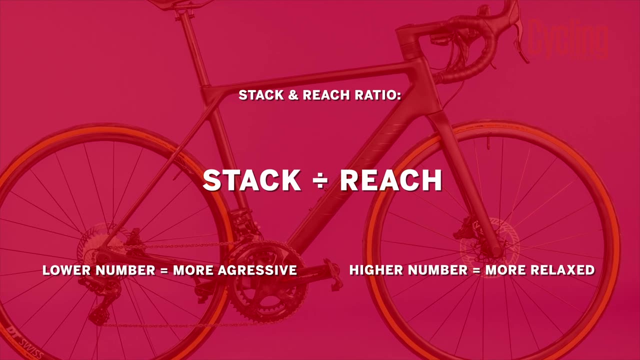 has a stack of 555 millimeters and a reach of 398 millimeters, versus a 56 centimeter specialized Roubaix at 611 millimeter stack and a 381 millimeter reach. Those are quite notable differences. So some people like to use stack and reach ratio. 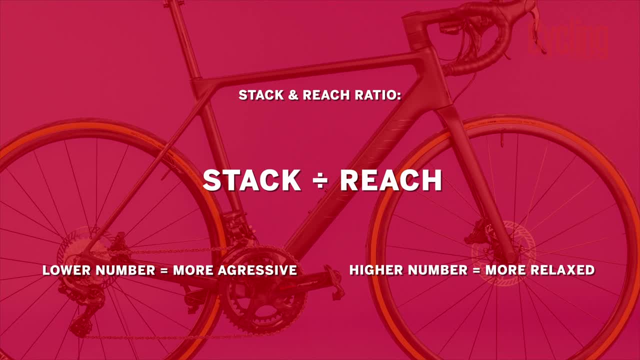 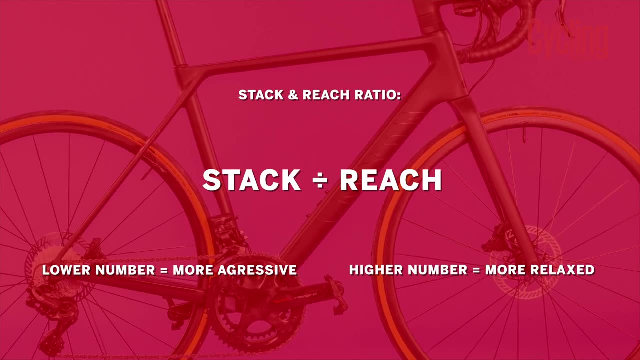 which is stack divided by reach. As a rule of thumb, a lower number is gonna be more aggressive and a higher number is going to be more relaxed and comfortable. It sounds perfect, right, But there are caveats to bear in mind. Stack and reach does not take into account. 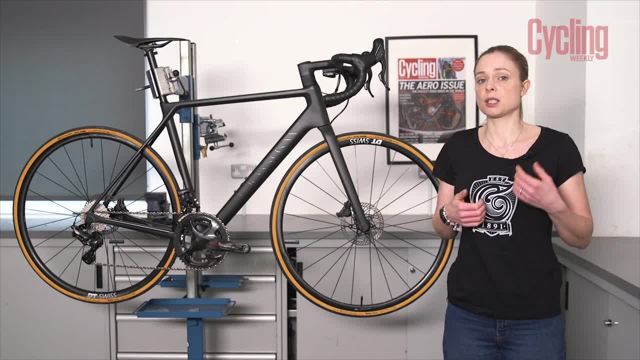 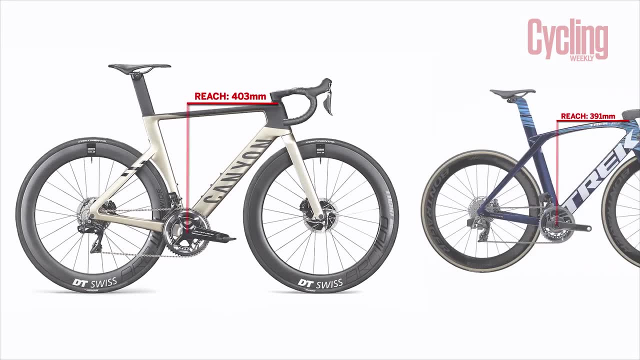 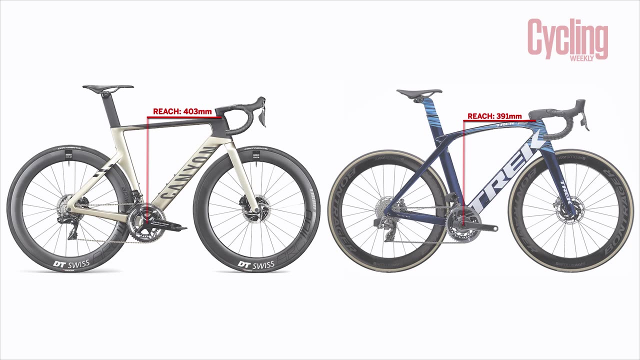 various different components on the bicycle, For example the stem length and also handlebar reach. A very good example of this is the difference between a Canyon Aeroad and a Trek Madone in H1.5 fit. The Aeroad in a large comes with a reach of 403 millimeters. 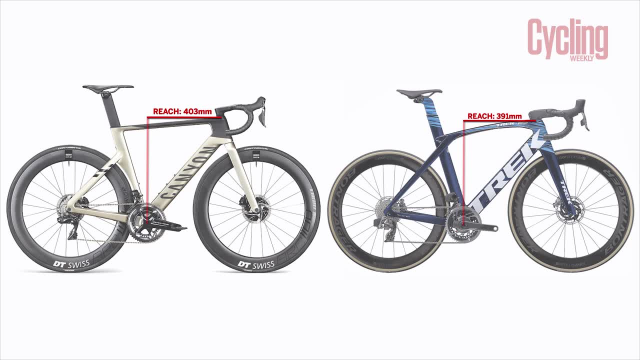 versus the Madone's 391 millimeters in A56.. However, the Madone uses a much longer reach handlebar And that is a factor that would not be immediately obvious from the geometry chart. You can often see the handlebars reach if you actually go to the spec sheet. 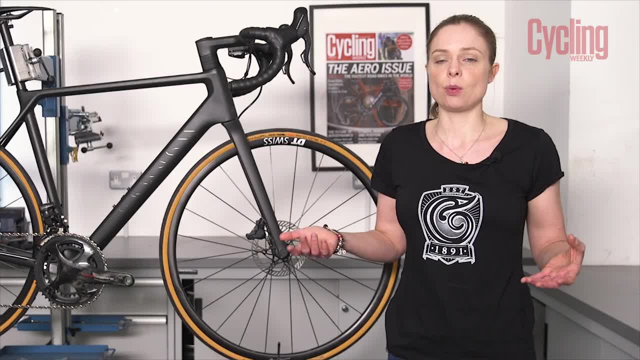 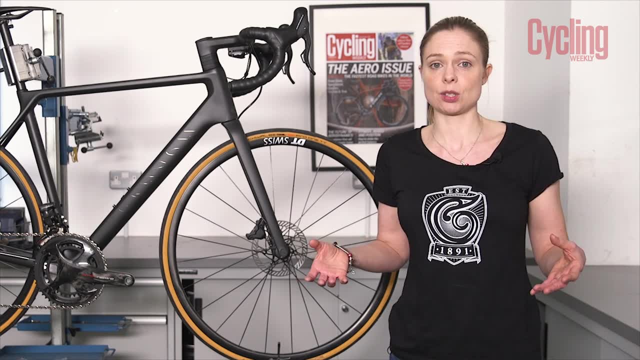 for that particular component. Alternatively, at that point you are looking at speaking to bike fitters or also calling in a test bike, which is something I always, always recommend if you're really looking serious, Seriously investing in a new bike. 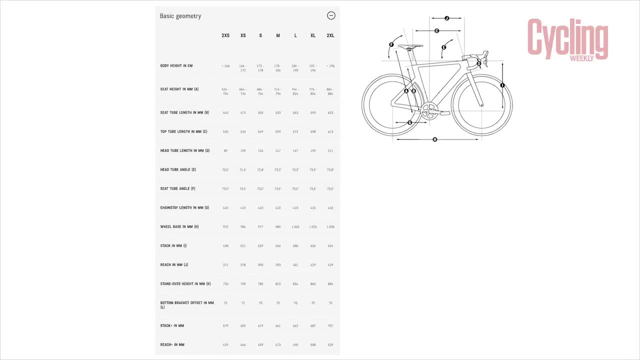 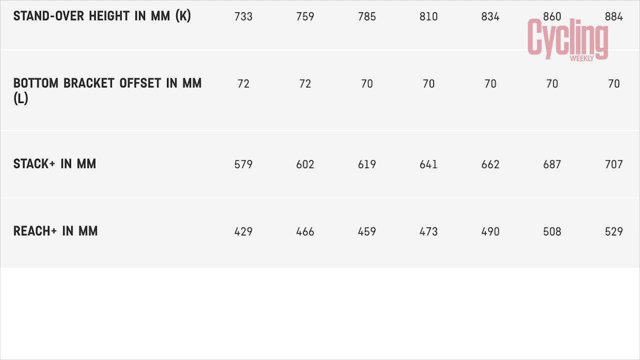 So, thankfully, some brands are actually starting to take this into account. For example, Canyon has started listing stack plus and reach plus, and that does take into account the stem and also handlebar reach. Do remember, though, that you need to look at the bike. 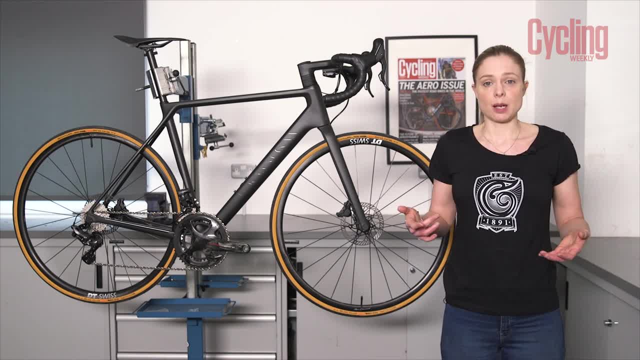 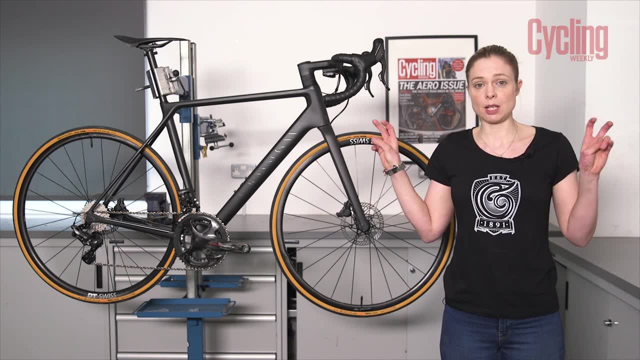 in your specific size. That is because, at times, bike designers will make the bike more or less aggressive in smaller or larger sizes, using the middle size as a median or average. This is often a cost cutting method because it allows them to use the same mold. 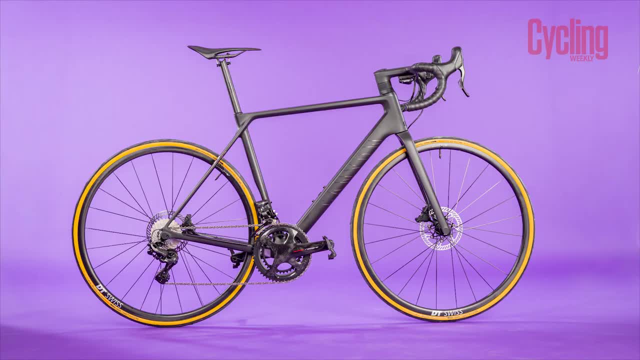 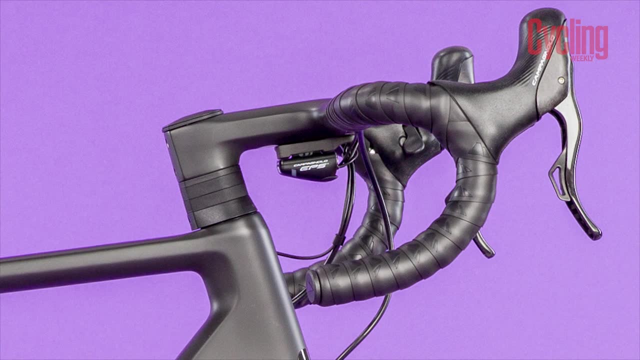 for various parts of the frame across different sizes. So one final thing that you should also bear in mind is that stack and reach does not take into account the effect of spaces, So if you are running all of the spaces below your handlebar, it will bring the stack up. 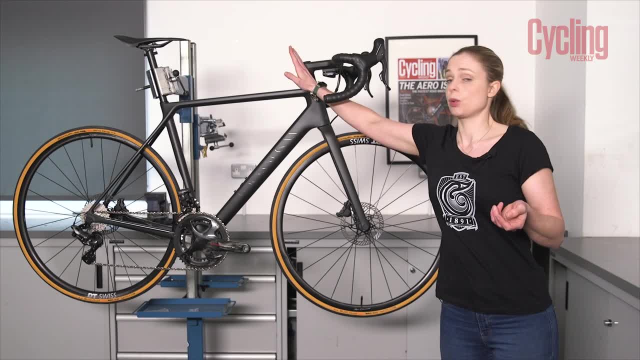 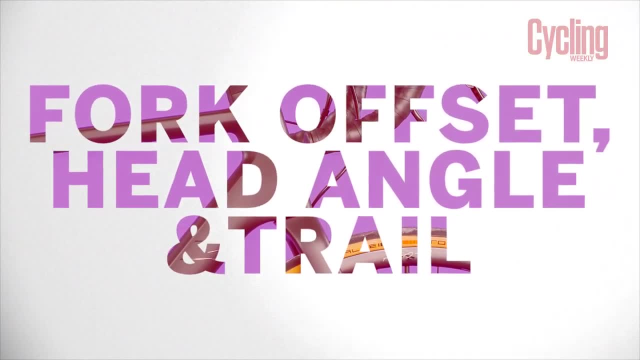 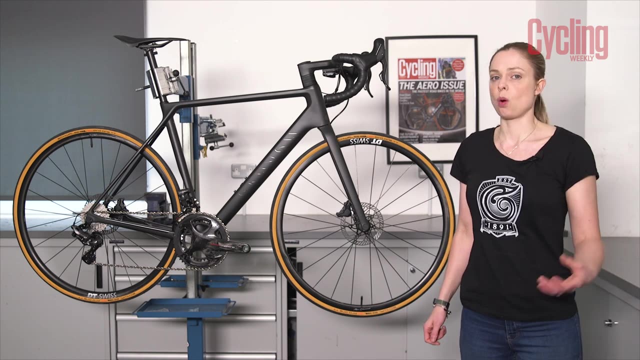 and it will also bring the reach very slightly back, because of course you've got a diagonal line here. Fork offset, sometimes called rake trail and head angle are intrinsically intertwined. It's quite impossible to look at one without looking at the others. 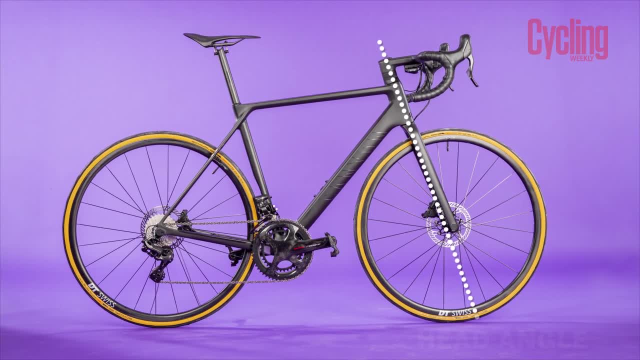 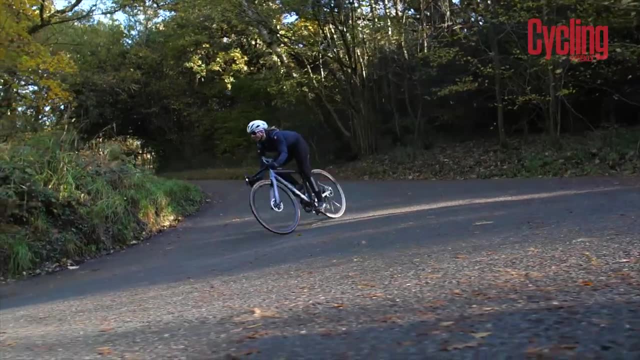 So head angle is the angle at which a line would travel through the head tube to the steering axis to hit the floor. Steeper head angles will handle more quickly. It'll take less input from the rider in order to get that bicycle to turn quickly. 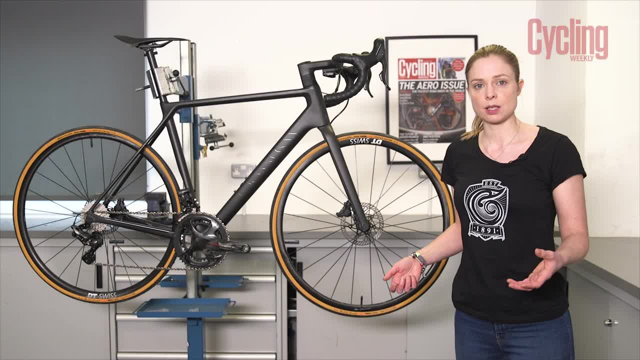 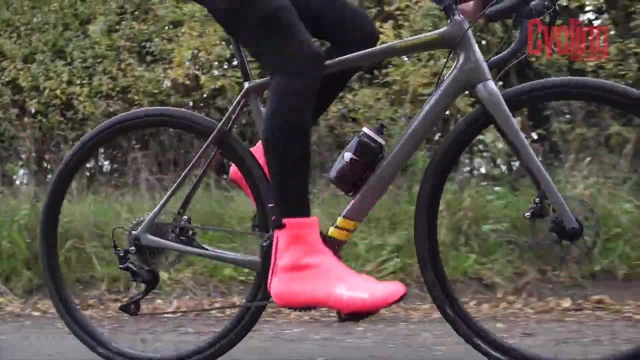 However, they can feel a little bit twitchy at slower speeds, Whereas a slacker head angle will feel a little bit less nippy and a little bit less twitchy when traveling at fast speeds, but will feel more stable at slower speeds. 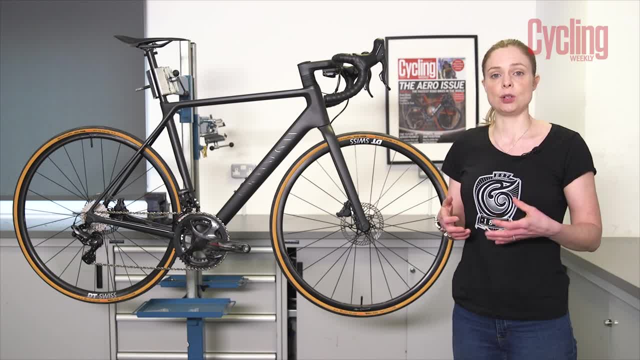 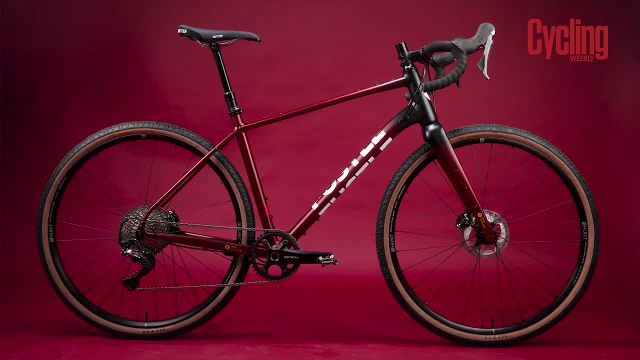 So this is a really interesting one to look at when we're talking about the new crop of gravel bikes, because it will really show you whether this bike is tending towards the mountain bike end of the spectrum or more towards the road bike end of the spectrum. 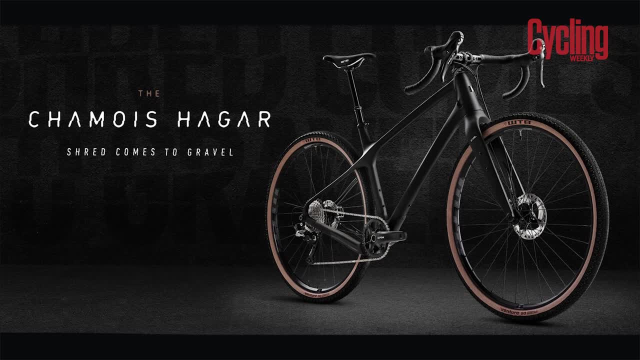 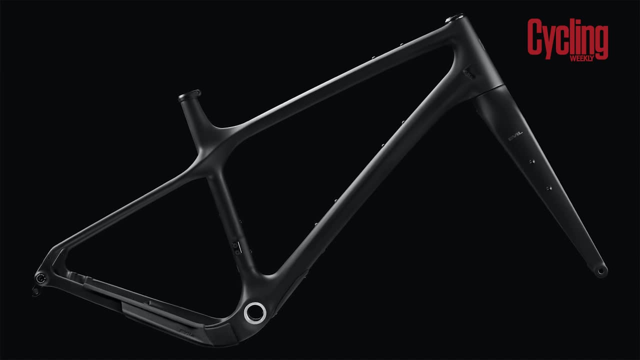 So the very perfect example of that is the Evil Shammy Hagger, which has a head angle of 60 degrees, 66.67 degrees. That is really, really slack And it's very much in the arena of mountain bikes Now on most road bikes. 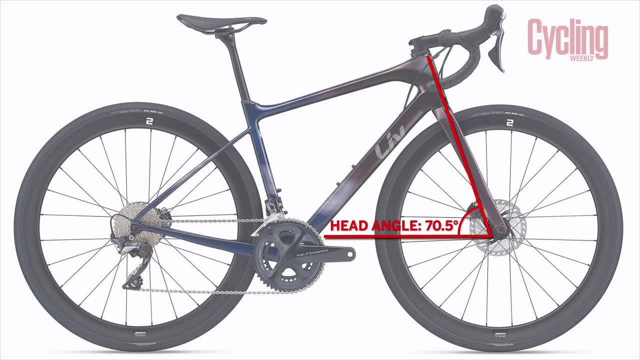 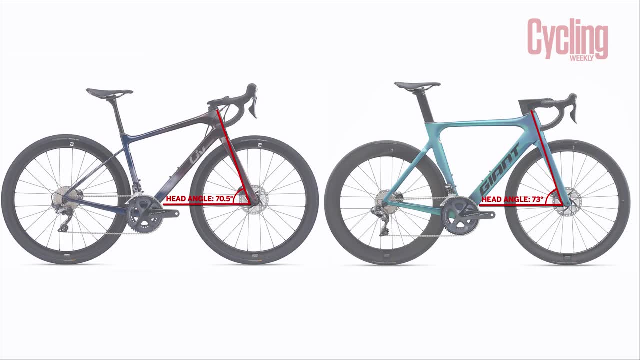 we would generally see a head angle of around 70 to 71 degrees as being quite relaxed and more in tune with a sportive or endurance bike, Whereas 72 to 73 degrees is something that you would see on a race bike. Those sound like really small differences. 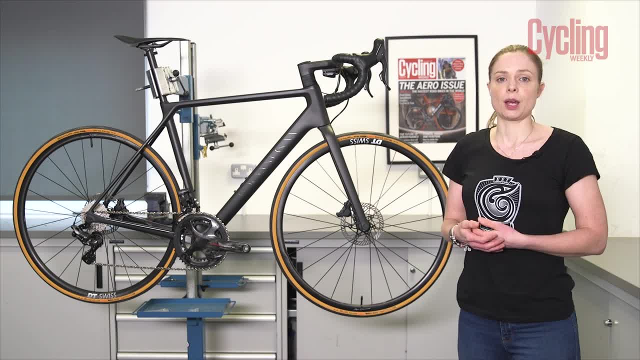 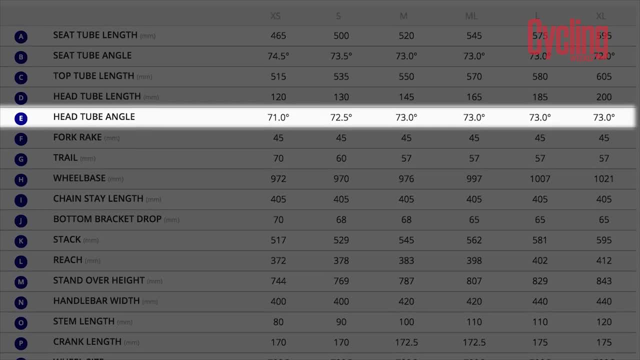 but they're definitely not, And they do make an incredibly big difference to the way a bike rides and handles. There is a caveat to this in that in very small bikes, sometimes we see the head angle becoming slacker in order to prevent toe overlap. 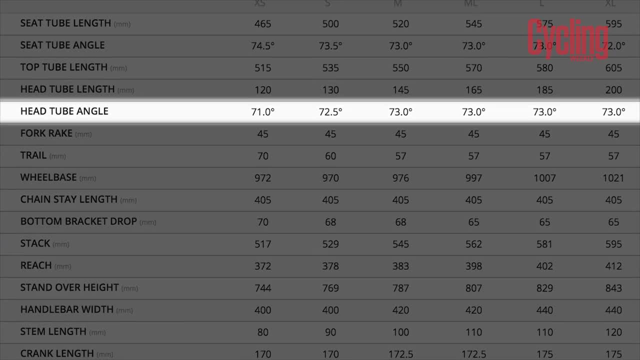 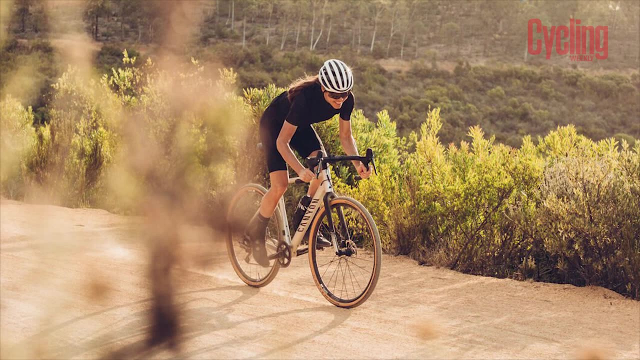 simply because the wheels are very large on the frame size. Brands have gone some way to counteract that. As an example, Canyon releases its much smaller women's bikes with 650B wheels. So offset or rake is how far the front axle is offset. 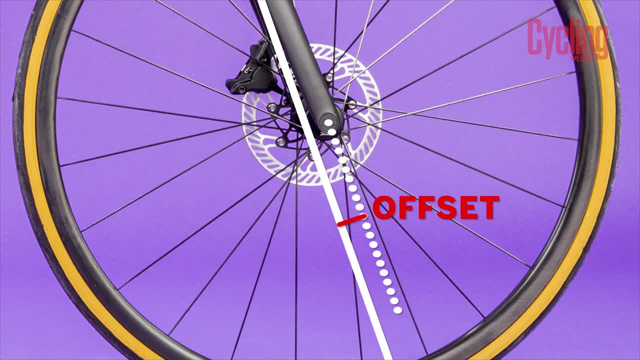 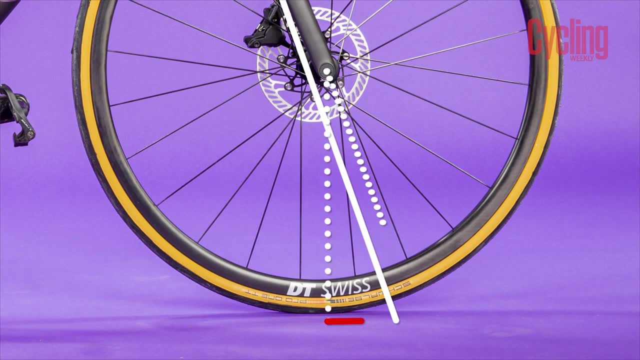 from the steering axis. Imagine a straight line from the center of the steerer tube to the ground. It's. the gap between that and the front axle Trail is the distance between the tire's contact patch with the ground and where the head angle hits the floor. 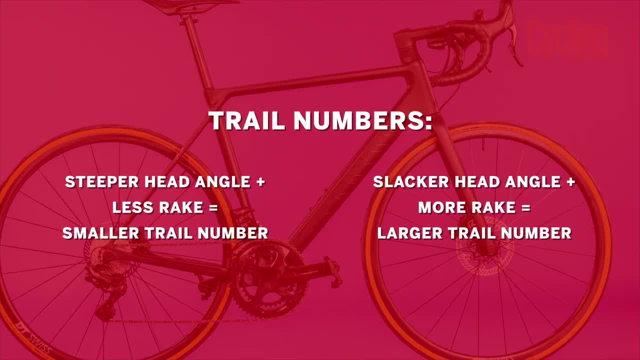 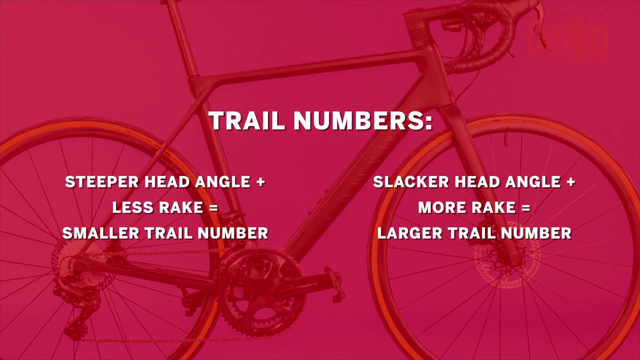 It's a product of the offset and head angle. So a short trail number is gonna involve a steeper head angle and less rake, Whereas a larger trail number is going to involve a slacker head angle and more rake. So, as a rule, 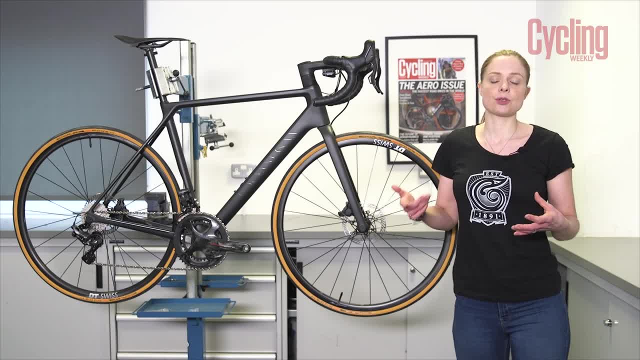 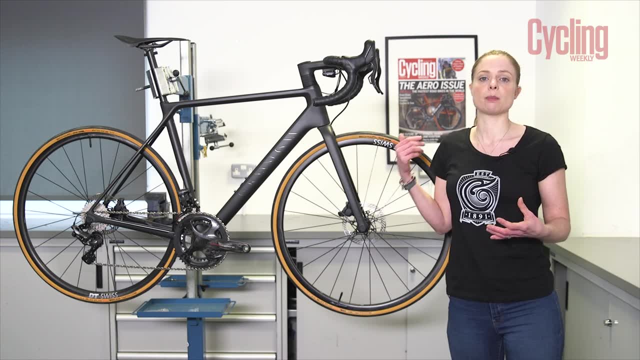 around 55 to 59 millimeters is the kind of trail that you would see on a fast, quick handling bike, Whereas 60 millimeters plus is more what you would expect from an endurance bicycle. So, as an example, Trexamonda in a size 56 has a trail of 58 millimeters. 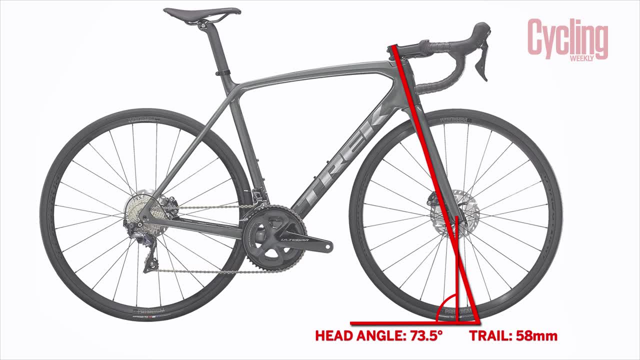 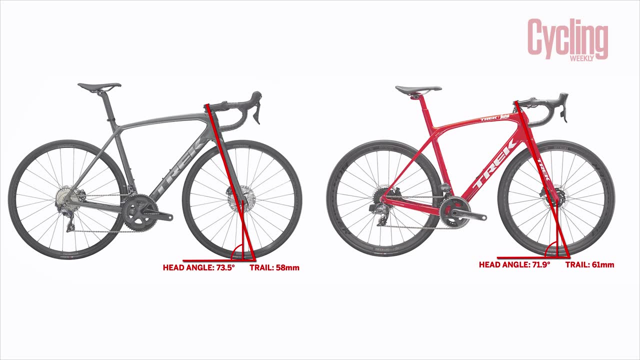 and a head angle of 73.5 degrees, And that, of course, is a fast handling race bike. Comparatively, the Domane has a trail of 61 millimeters and a head angle of 71.9.. And that is very much an endurance bike. 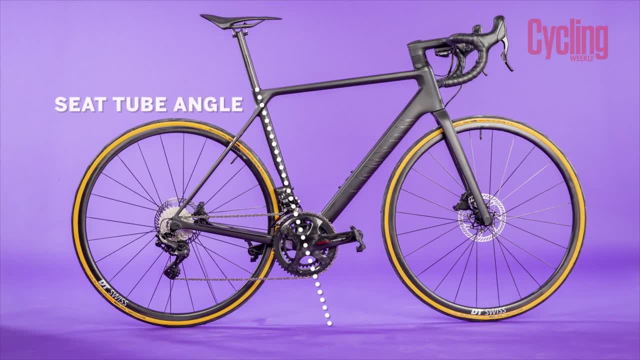 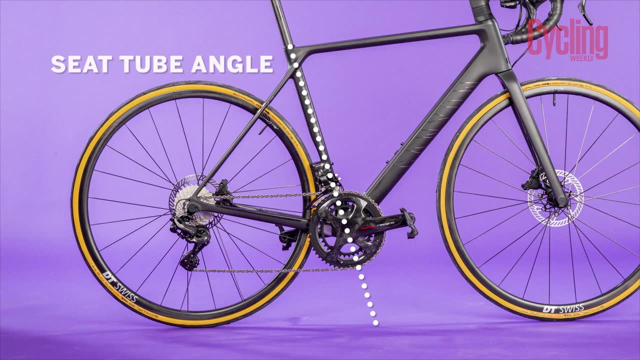 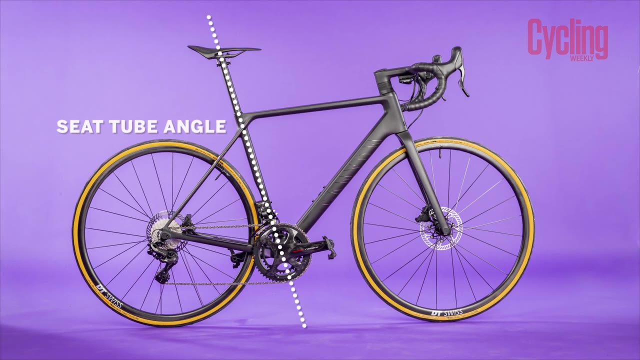 Another one to bear in mind is also seat tube angle. Now, in most road bikes this will vary between 72 to 74 degrees, And it generally remains fairly consistent across the sizes. This can actually represent a problem for taller riders, Because the seat tube is longer. 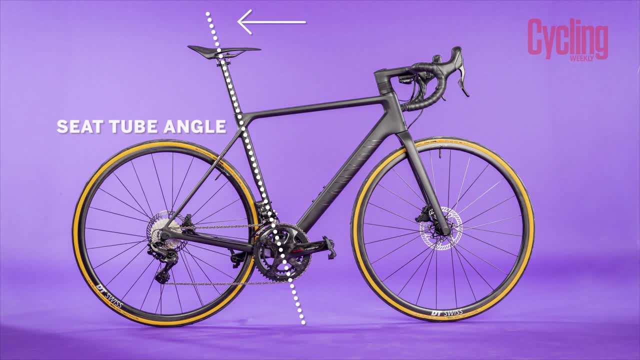 it means that the saddle is pushed further back. Of course you can push it forward on its rails, but it can only go so far. This means that the saddle is pushed further back. Of course you can push it forward on its rails, but it can only go so far. 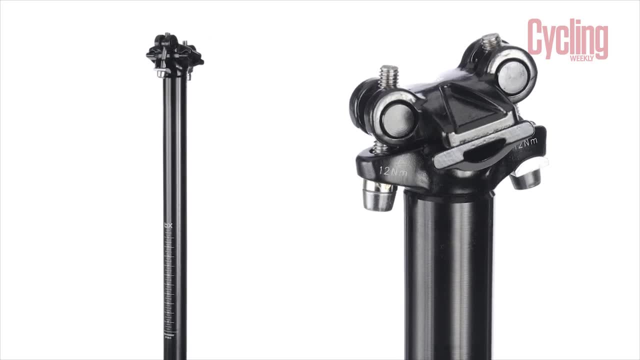 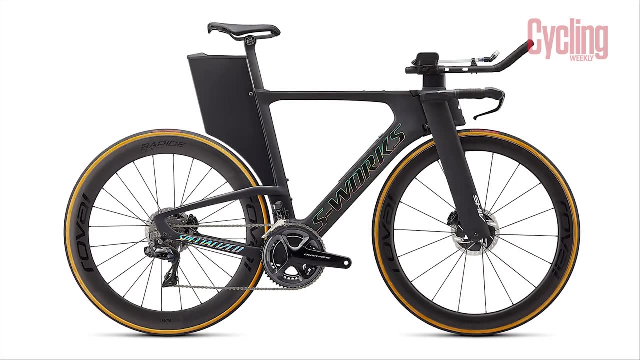 This can be counteracted with an inline seat post, and that can help to get the saddle further forward. However, it'll only take you so far, So if you want to understand what kind of effect that seat angle has, it's worth having a look at the TT bikes. 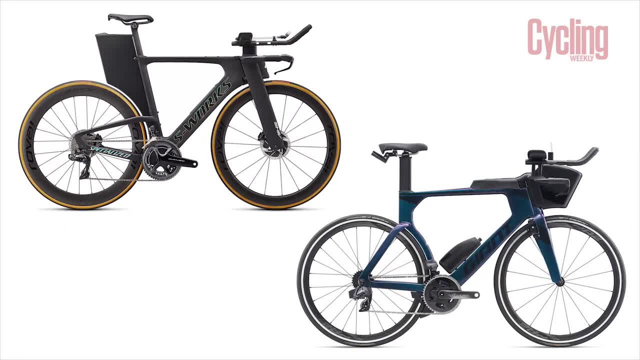 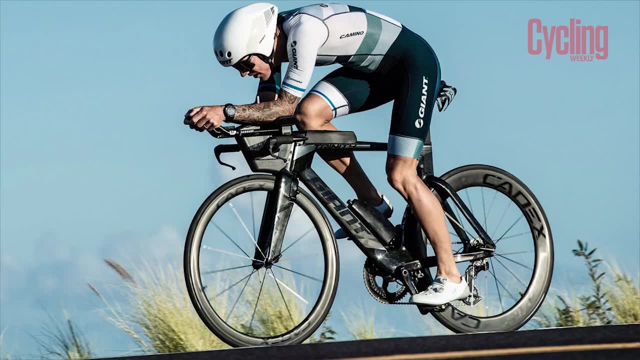 that you get on the market. So both the Specialized Shiv and the Giant Trinity have a seat angle of 77 degrees. That is much, much steeper and it will put the rider much further forward up and over the bottom bracket. 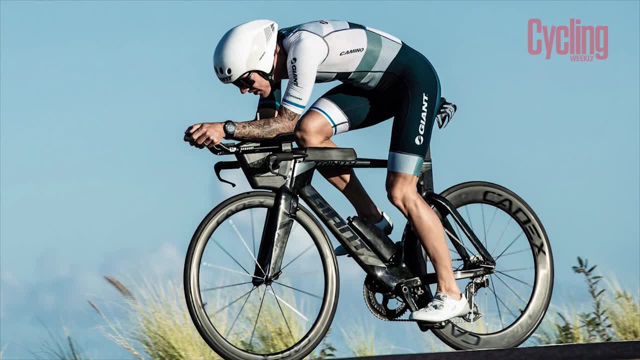 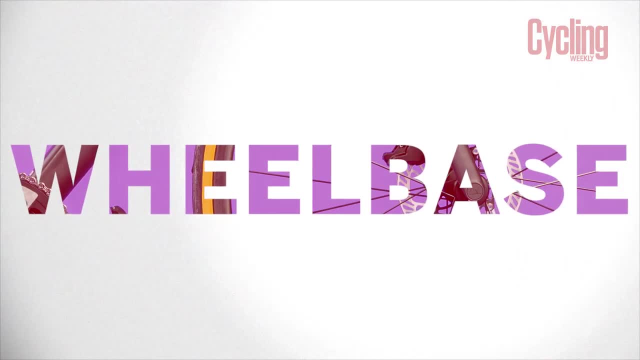 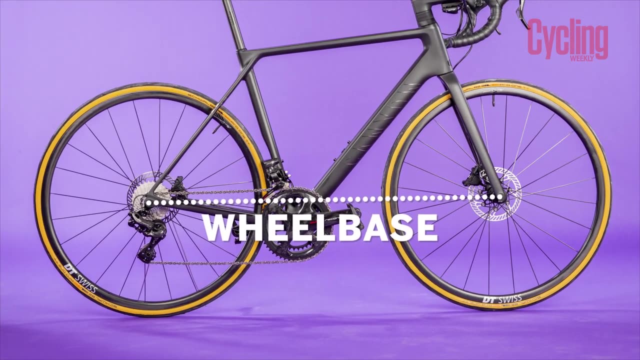 allowing them to get that fast flat back aerodynamic position and really to push the power through the pedals. Wheelbase is another marker of how quick-footed or stable a bike will feel. A longer wheelbase has a larger turning circle, whereas a shorter wheelbase has a shorter turning circle. 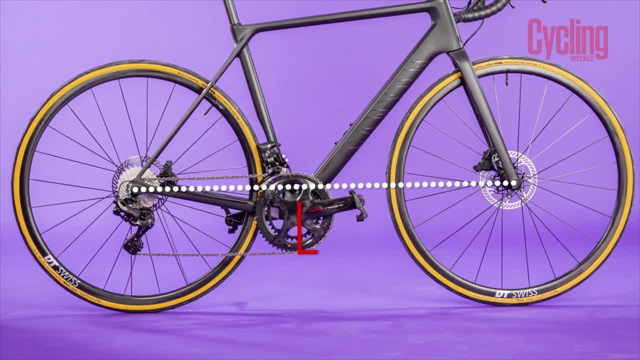 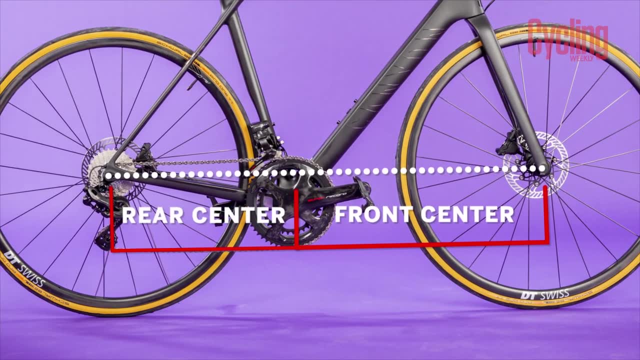 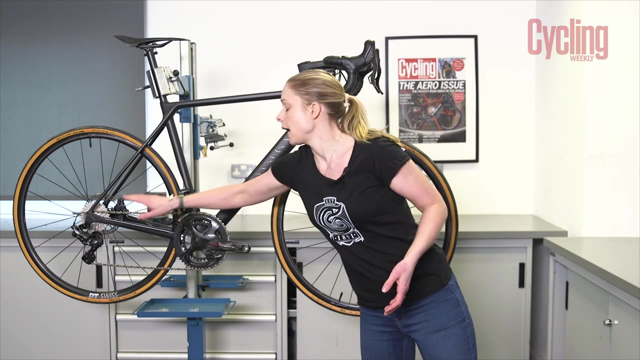 Wheelbase can be divided into: front centre- the difference between the centre of the bottom bracket and the front axle, and rear centre- the distance between the center of the bottom bracket and the rear axle. unfortunately, not all bike brands do list this. however, they do generally list chainstay length, which will of course give 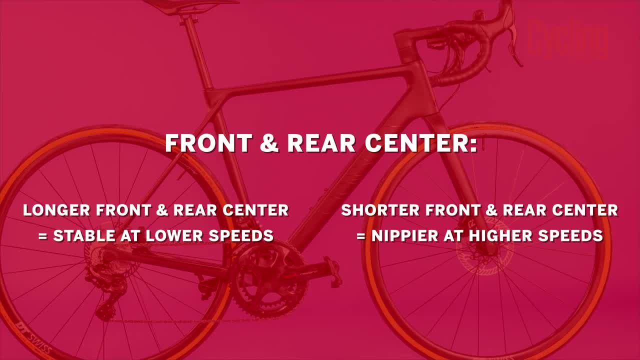 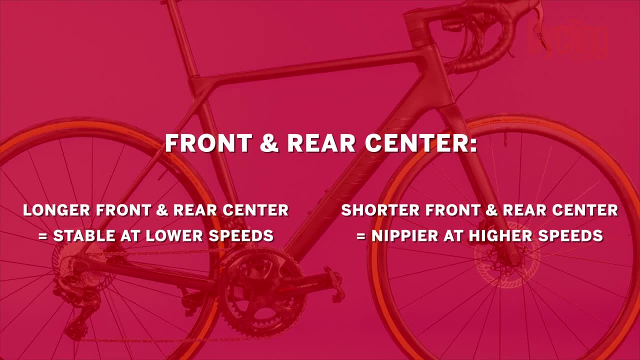 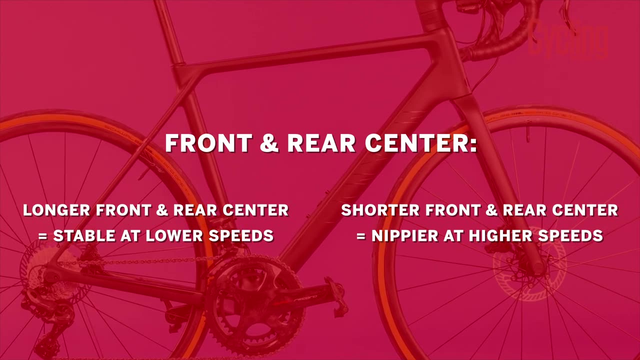 you a pretty good idea of rear center. so in both those cases a longer number. so a longer front center and a longer rear center will feel more stable at slower speeds, whereas a shorter front center and rear center or chainstay length will feel much more nippy if you're riding at faster. 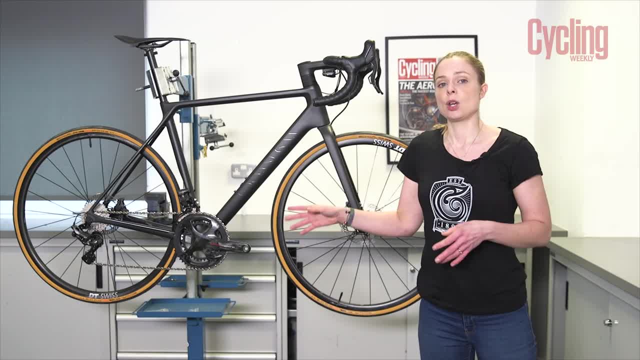 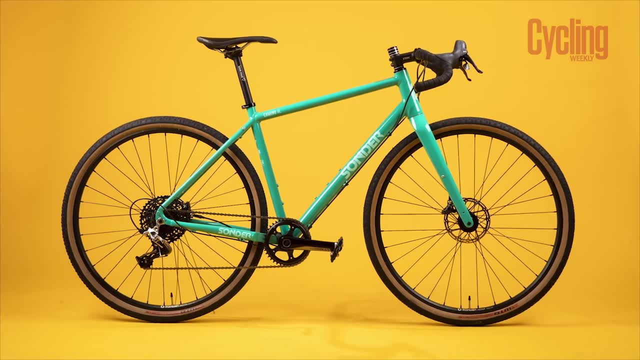 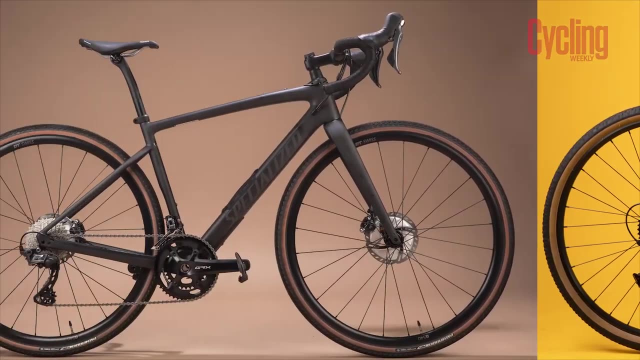 speeds. of course, the chainstays, or rear center, do need to be long enough to accommodate different tires, which is why often on gravel bikes, as well as them providing more stability, we also see longer rear ends, because this does allow for more tire clearance. however, there are some caveats to 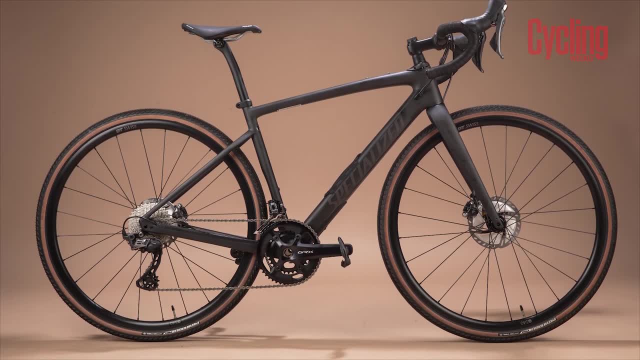 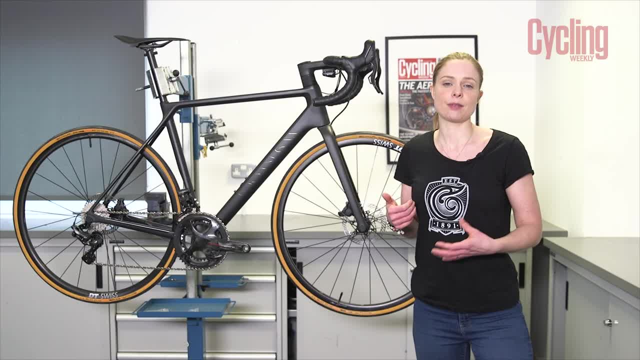 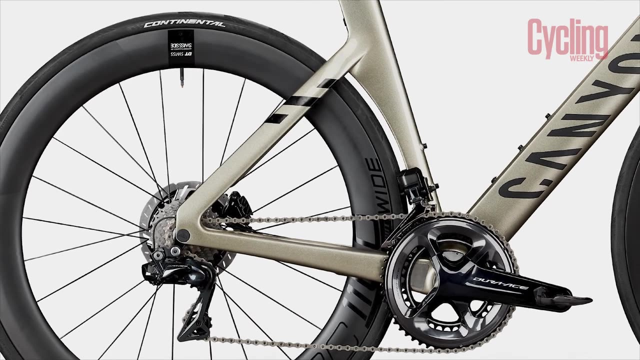 find off-road. so in the past disc brakes have interfered with this status quo. that's not the case anymore. group sets have changed so we don't need longer chainstays to account for disc brakes and we do see that in newer bikes. as an example, newest iteration of the canyon air road had 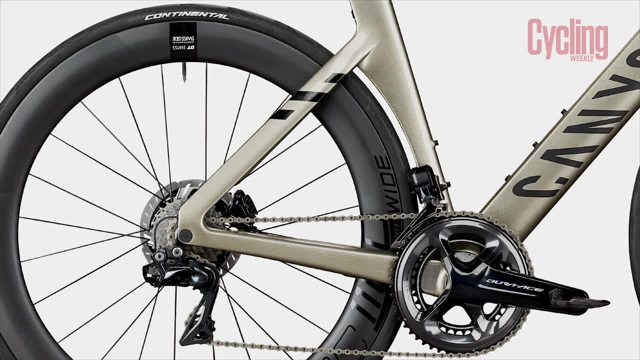 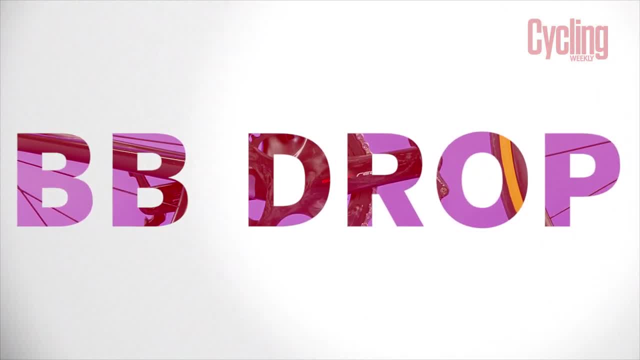 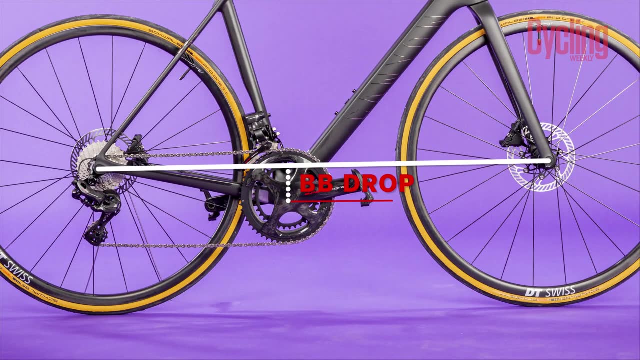 shorter chainstays again, which allowed it to keep its intended personality. so, last but not least, is bottom bracket drop. this is how far the bb drops from the two wheel axles. you can also look at bottom bracket height, which is the bb height from the floor. however, this is 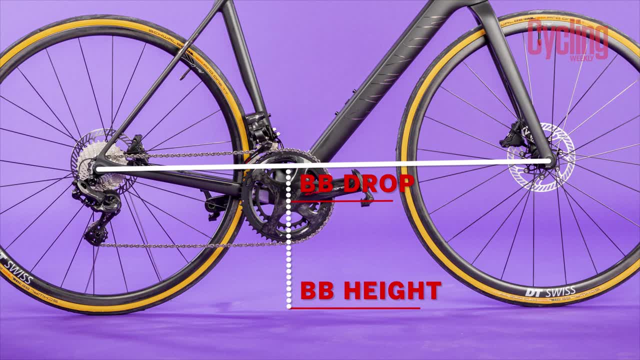 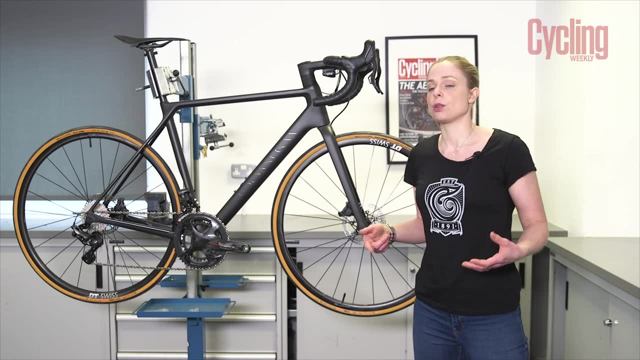 influenced by tire volume, so i tend not to focus on it quite as much. so a larger bb drop lowers the rider's center of gravity. it's something you would still want on a fast handling crit race bike, because you are going to be leaning hard into those corners and you want a. 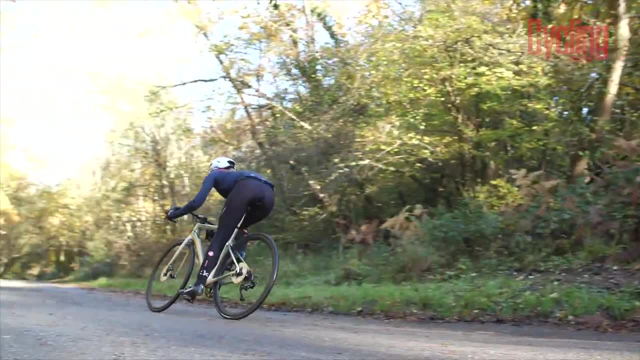 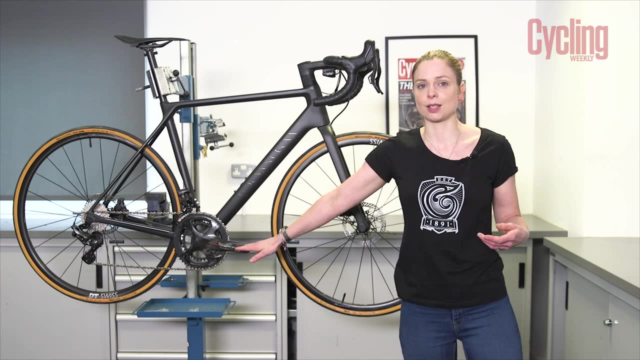 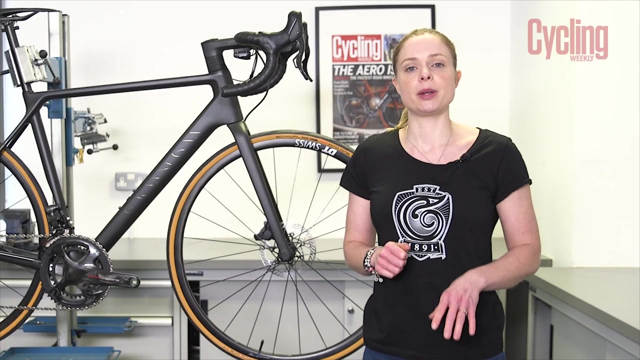 low center of gravity. the problem is if you go too low and you've got problems with pedal strike when you are leaning over into the bends and pedal strike can have some pretty nasty consequences, i can tell you. it's also a key measure that we look at when we're looking at off-road bikes. 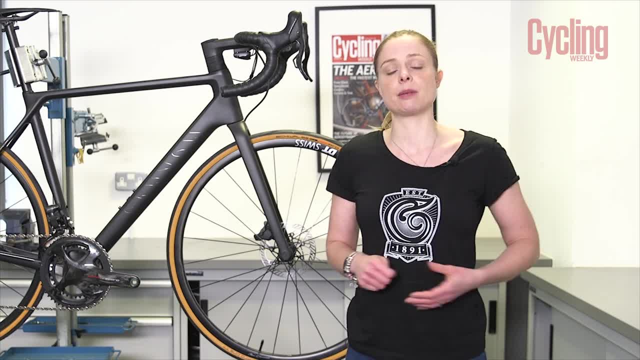 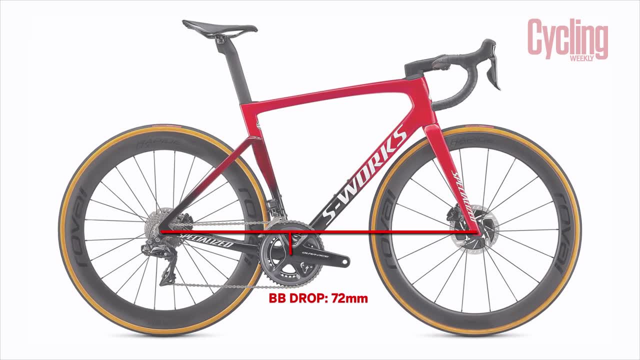 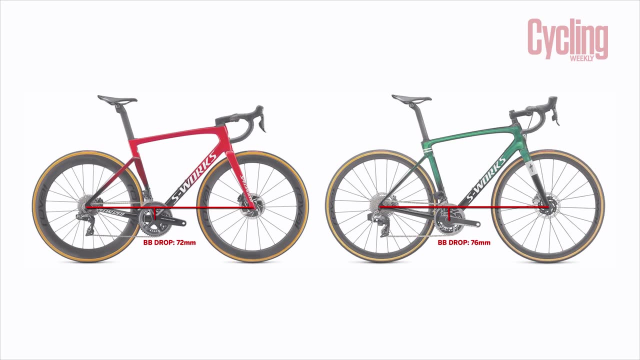 because, of course, pedal strike and also clearance is something that becomes really, really important. so, using specialized as an example, a 56 centimeter specialized tarmac has a bb drop of 72 millimeters versus 76 millimeters on the specialized roubaix. however, on the cyclocross bike in the same size, 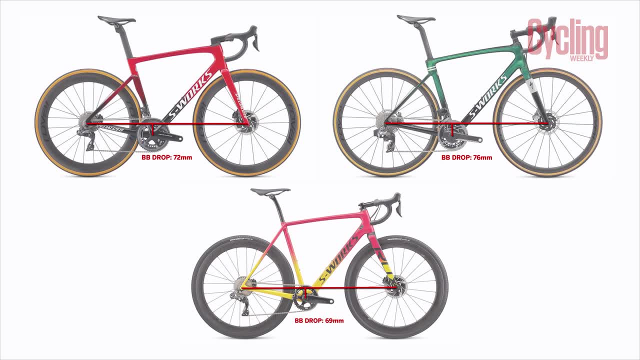 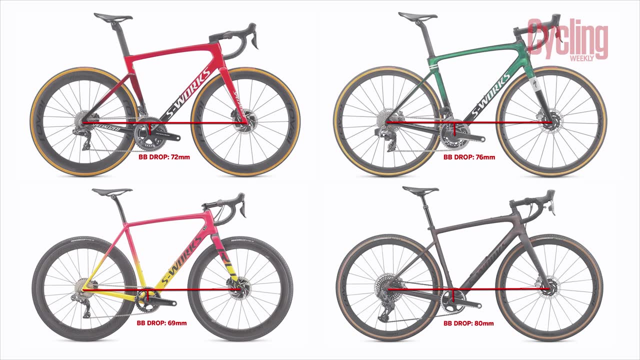 so still a 56 centimeter frame. it's 69 millimeters on the crux cross bike. however, on the diverge, it's 80 millimeters. now, that is a really, really big difference. it's going to make the diverge feel an awful, awful lot more safe and it's going to make the diverge feel a lot more safe, and it's going to 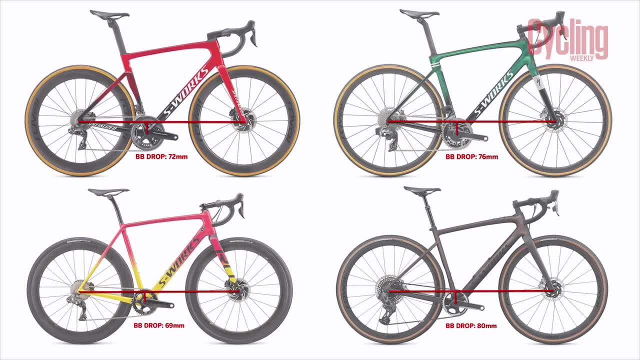 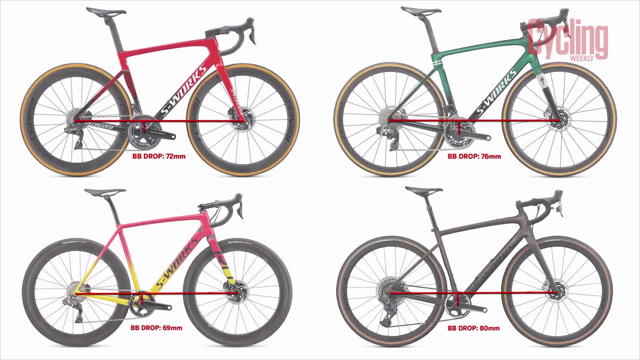 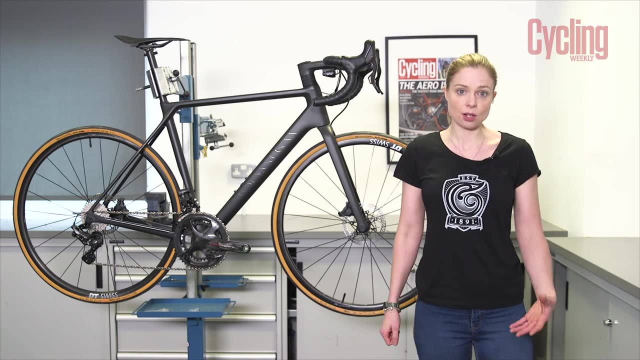 stable on gravel terrain. however, it gives you a lot less clearance, whereas the cyclocross bike is much more tailored to that really thick mud and obstacles that you might find on a cyclocross course. so there you have it. i've tried to cover off the key metrics that you need to look at when 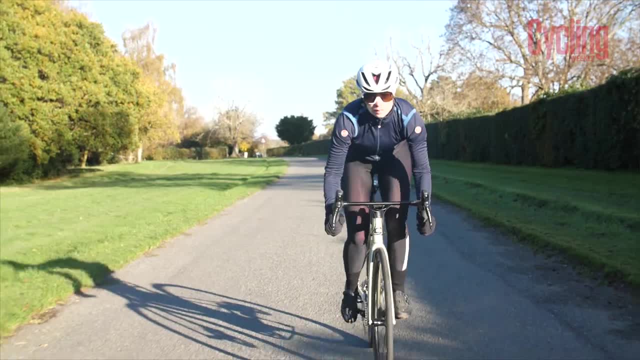 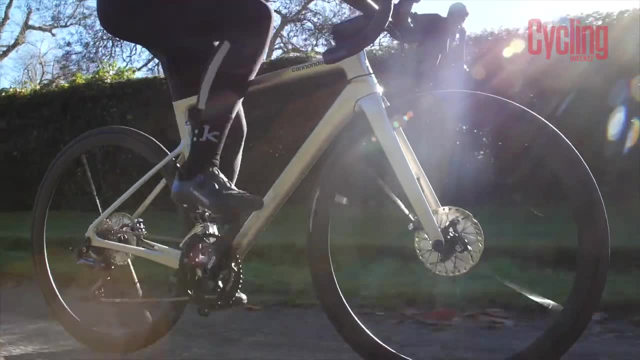 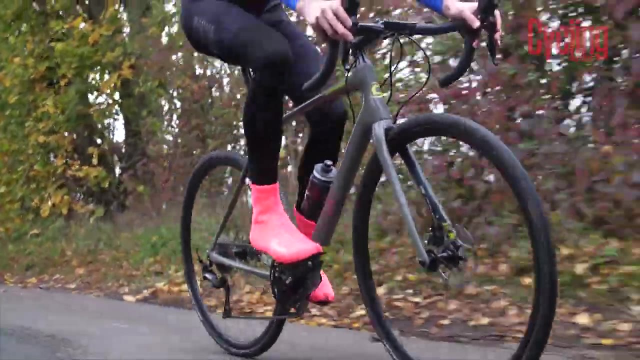 you are considering buying a new bike. in short, if you're after a fast, aggressive bike, then look for a long reach, a short stack, a steep head angle and a shorter trail length number. alternatively, if you're after a comfortable ride in a more endurance position for those long